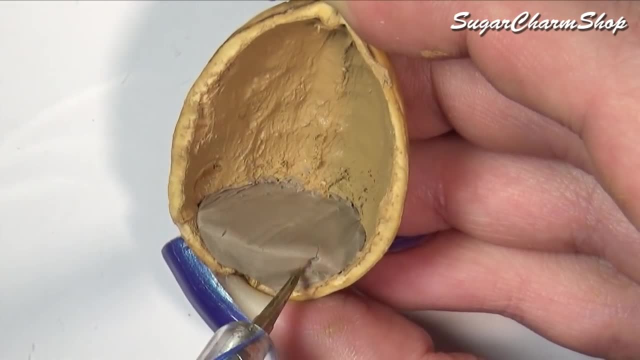 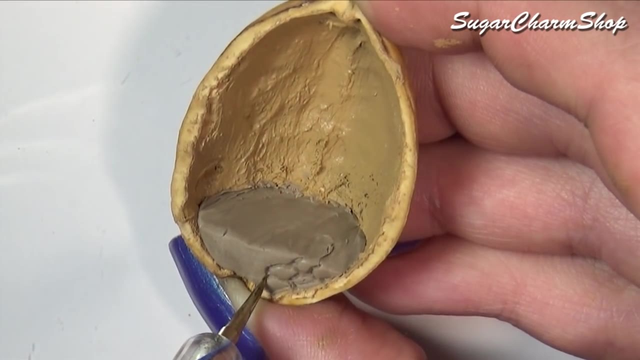 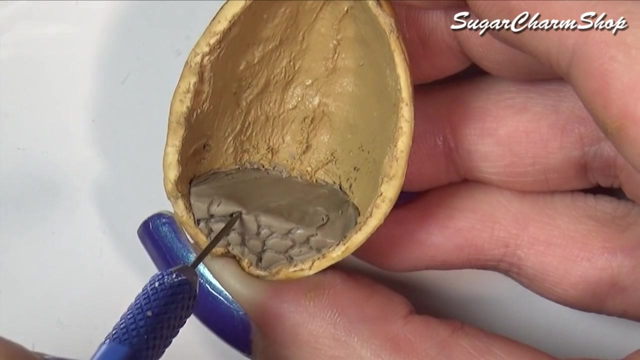 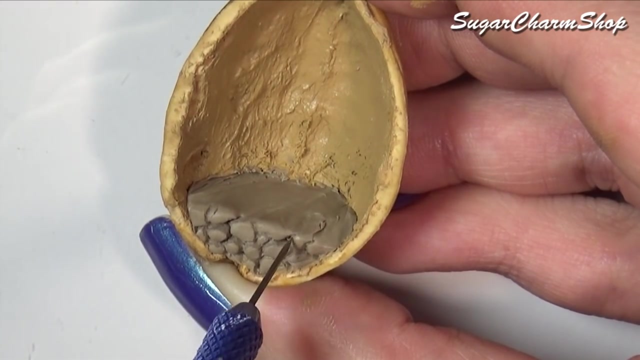 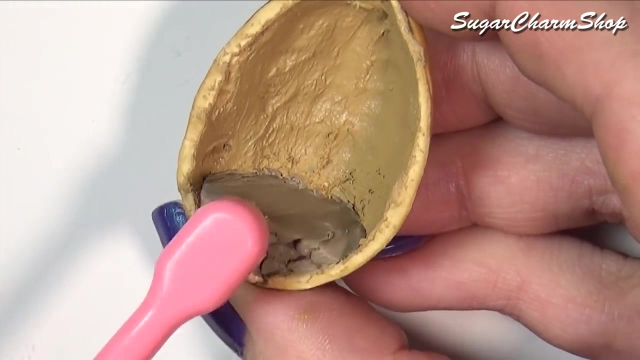 I first added some texture using a pointy dotting tool, then added texture to some of the rocks or pebbles using a needle tool. I then went in with some tin foil and a toothbrush. With this IComplete the walls. Add some light tan clay on top for the wooden floors. 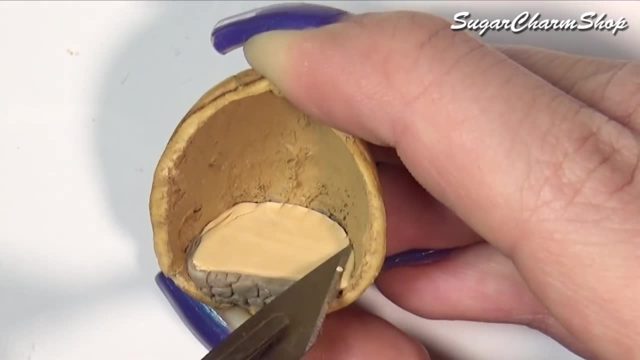 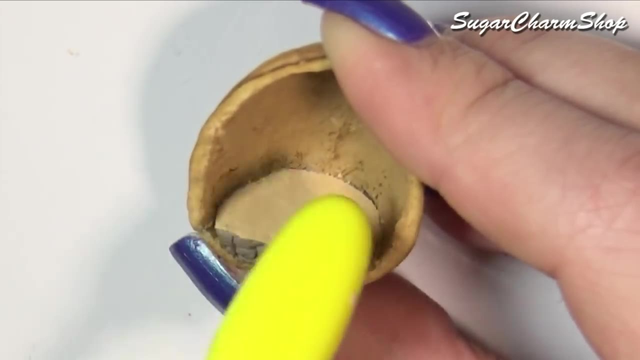 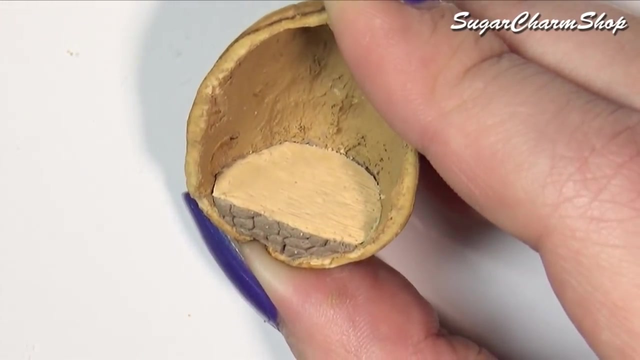 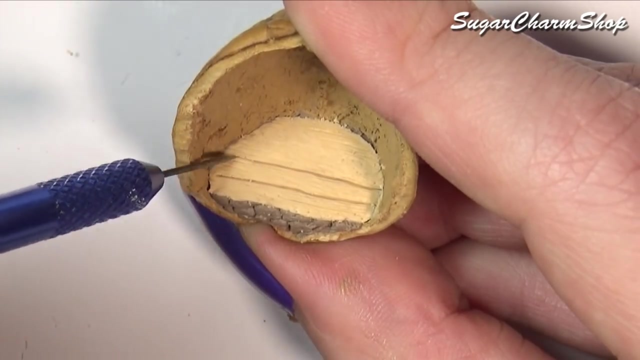 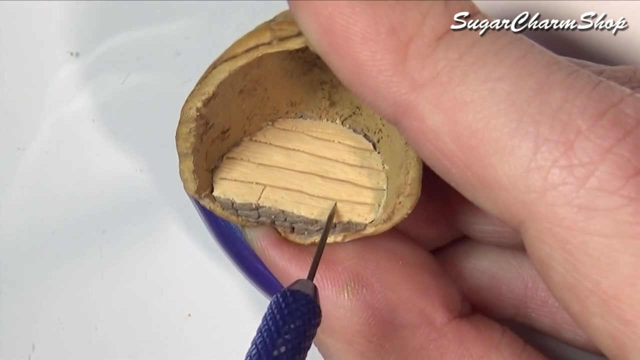 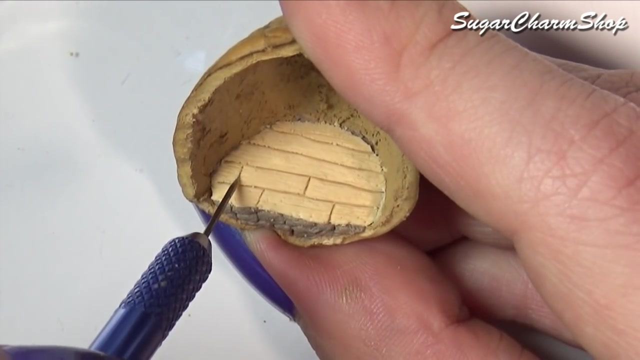 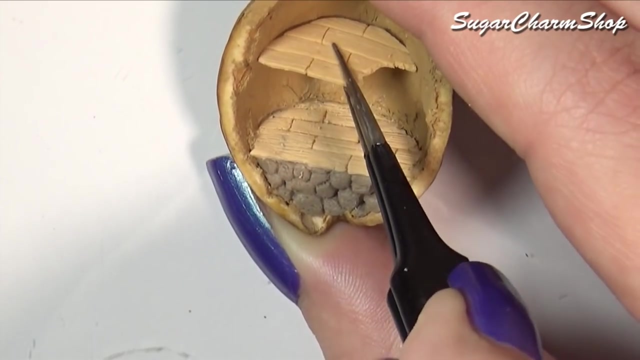 and add some texture using a toothbrush and a needle tool. I made and pre-baked another piece for the second floor or platform. I attached this using some liquid clay to hold it in a bit more securely And then baked the walnut shell. 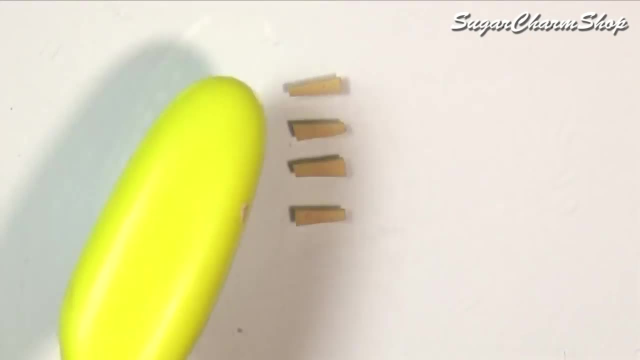 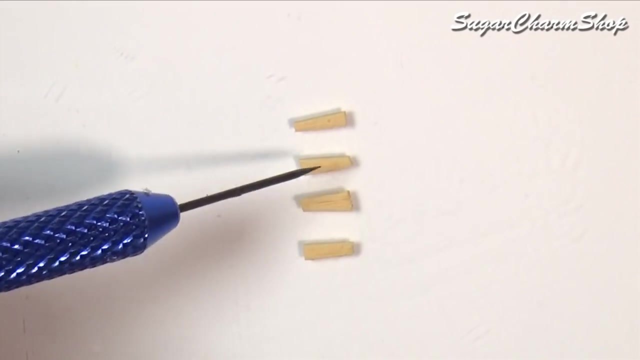 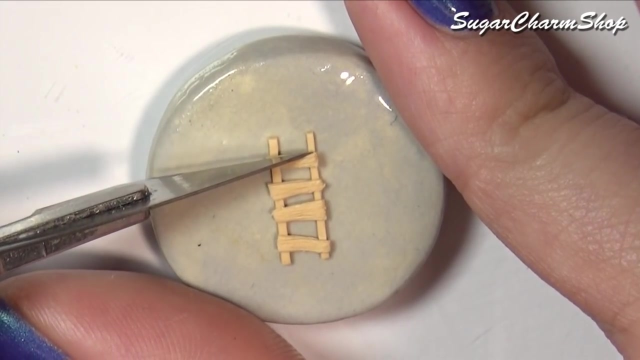 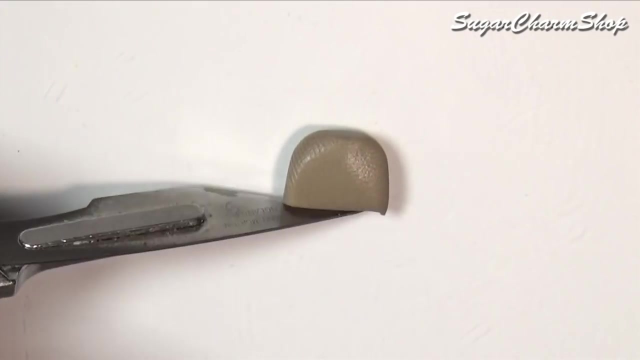 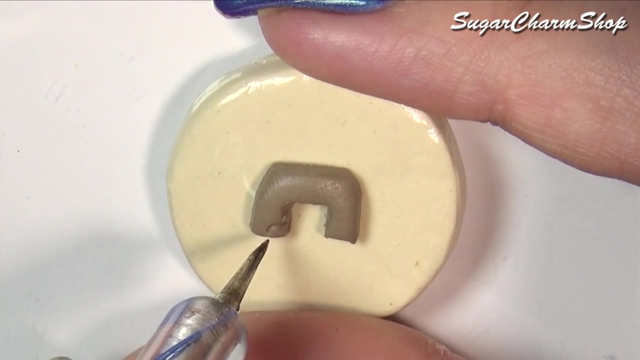 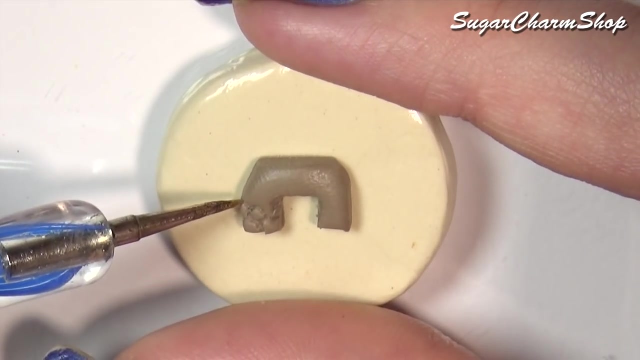 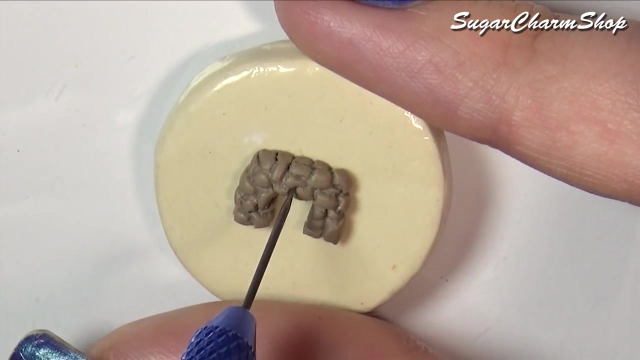 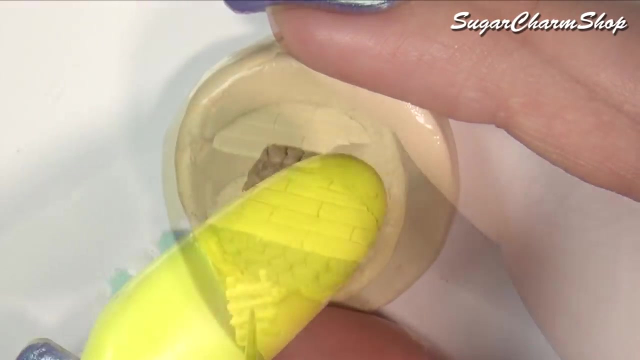 I made a tiny ladder and added some texture, using the same technique as for the floor, And I made a fireplace, adding texture the same way as with the foundation: Bake both pieces and glue them in place, and then use acrylic paint to paint the walls. 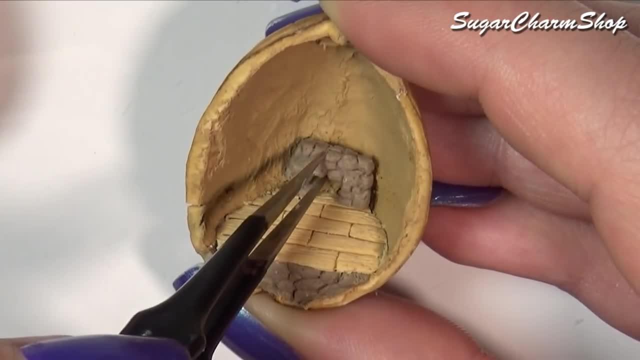 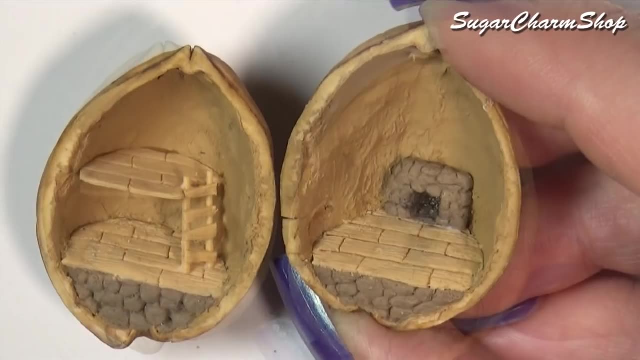 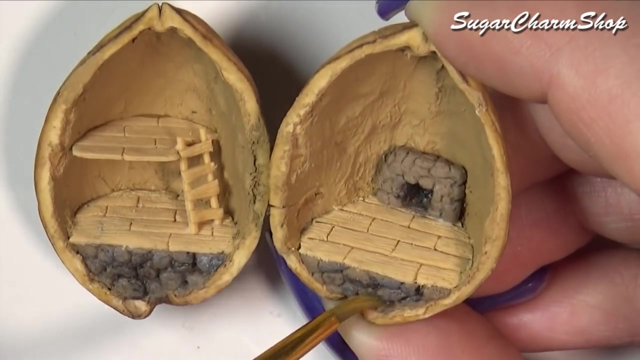 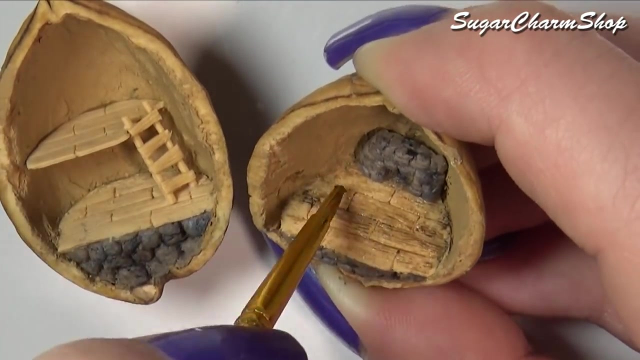 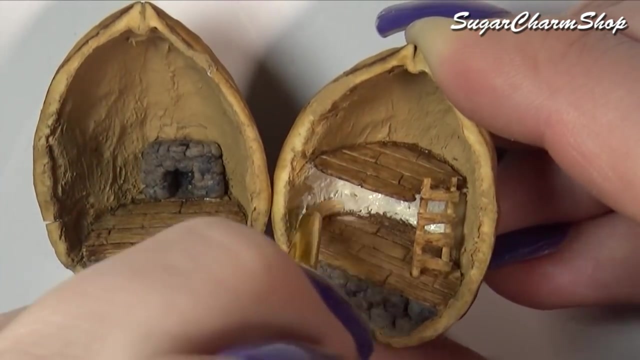 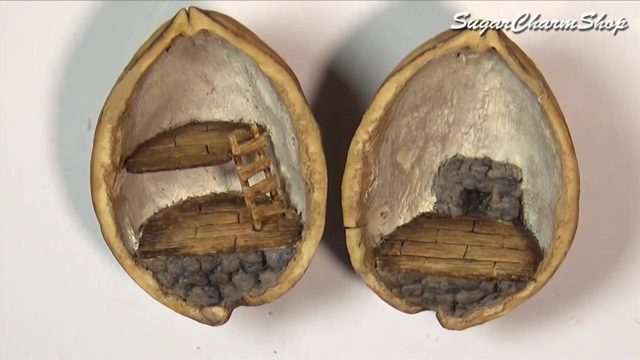 Bake both pieces and glue them in place and then use acrylic paint to paint each. This is by Richard Carpenter and is one of my favorite pieces of art. Looks great, everything you've made so far. I used brown clay to make some tiny twigs for the fireplace, baked that and added a. 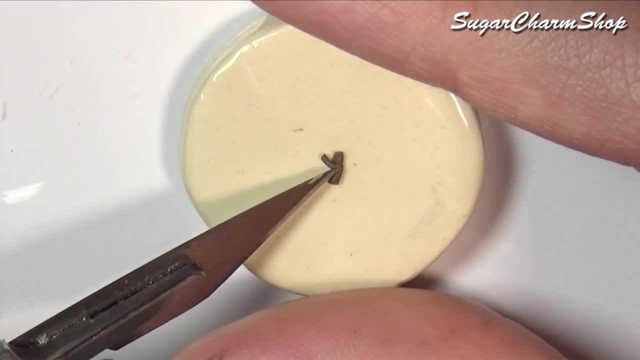 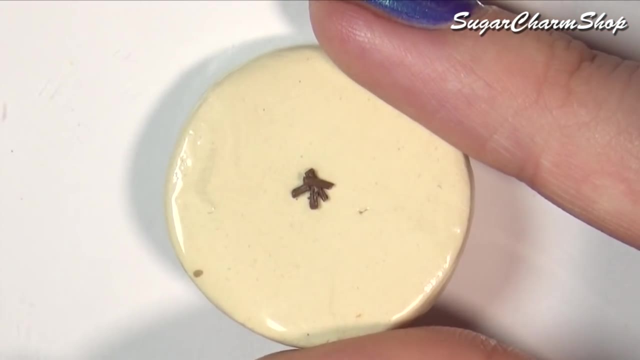 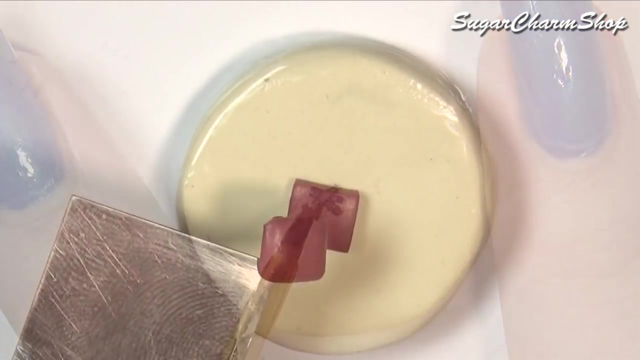 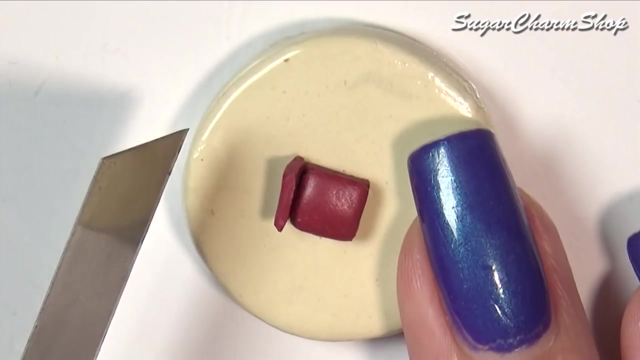 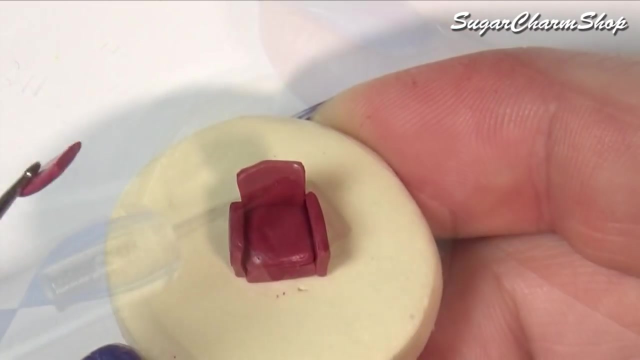 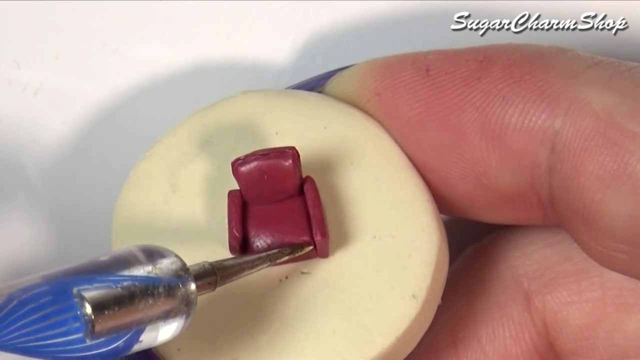 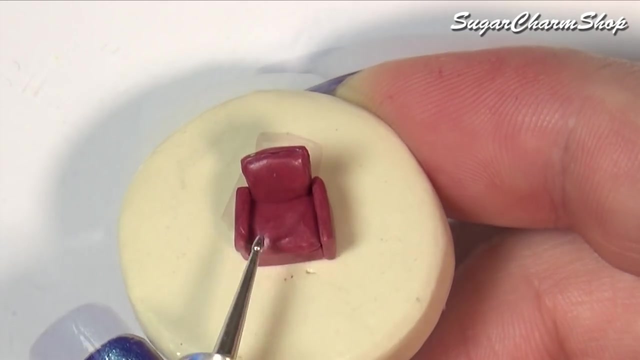 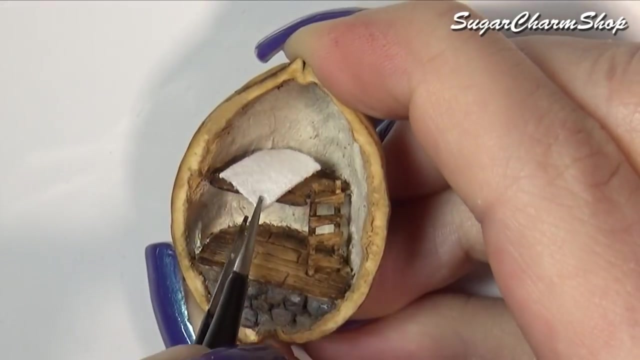 tiny bit of acrylic paint. I also used some black acrylic paint. I also used some dark red clay to make a chair, And for this one you want to use a toothbrush to add a tiny bit of texture before baking. Instead of making a bed, I just glued in two types of fabric. 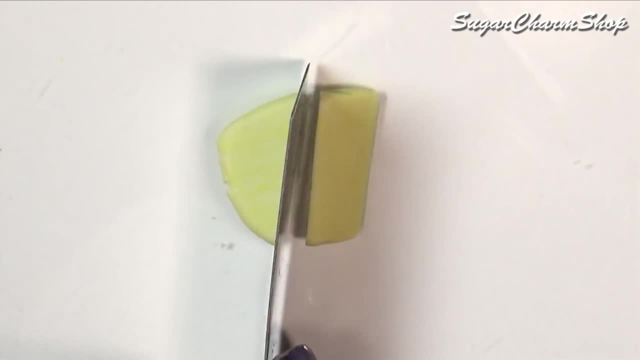 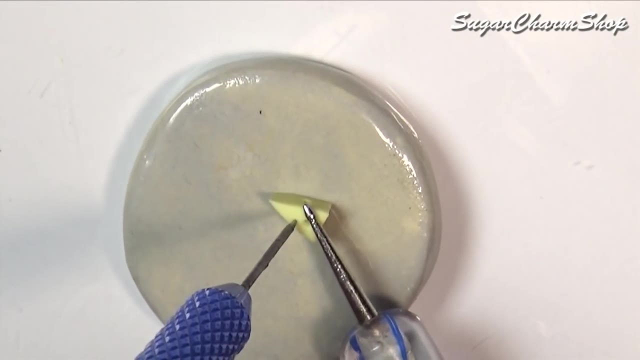 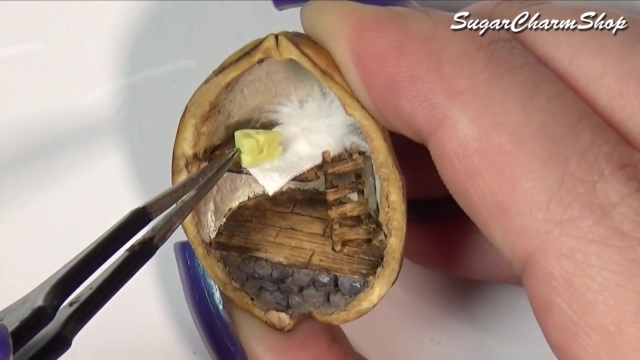 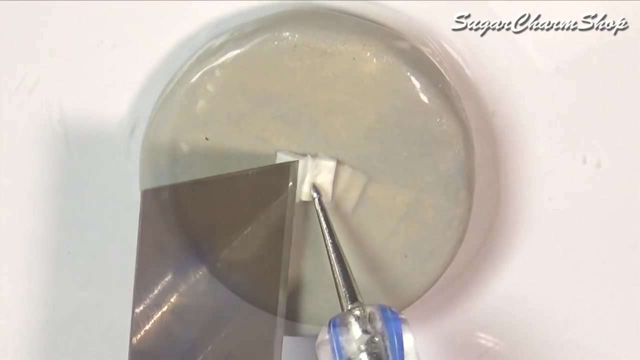 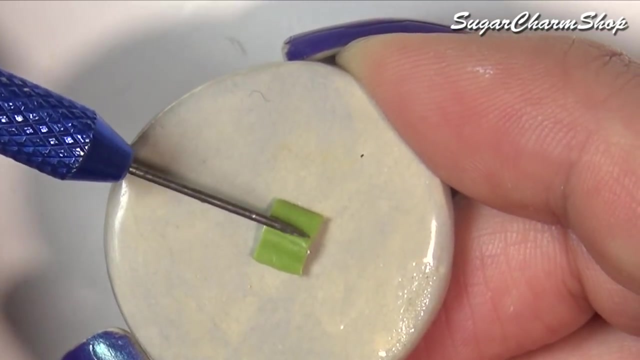 And then, of course, no mouse house is complete without a midnight snack. Last item I made, as far as the decor goes, is just a simple book, And for this one I started out by making the pages, then added the binding, used a needle tool to add a few details, then baked that and painted it using acrylic paint. 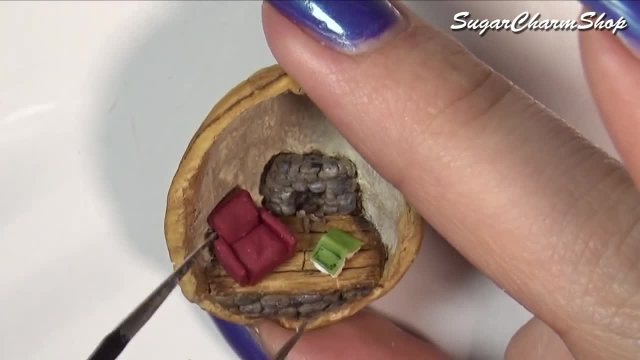 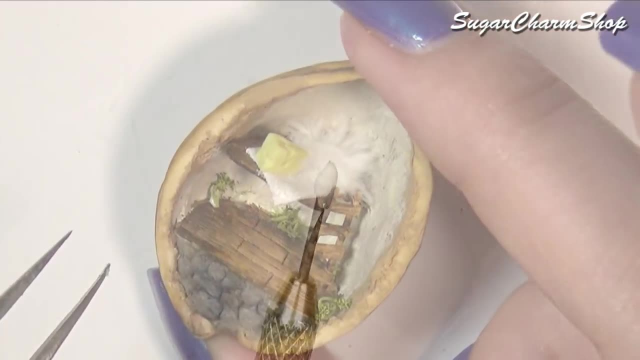 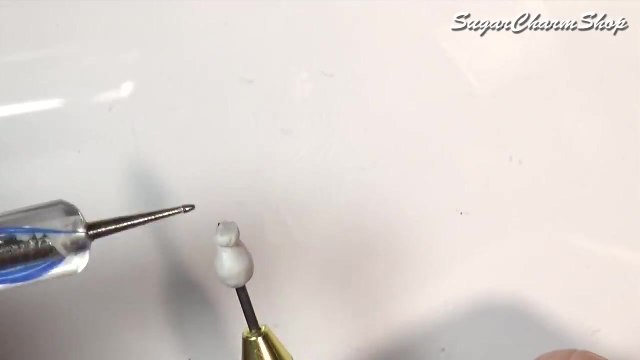 And finally, I just glued in a tiny bit of preserved moss. Lastly, we are going to be sculpting the mouse itself. For this one, I first added some clay to the tip of needle tool and then pre-baked that to have a nice base for sculpting.